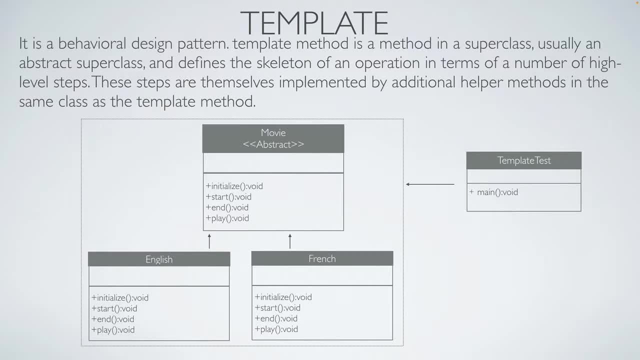 Today we are going to talk about template design pattern. Template design pattern is a behavioral design pattern. Template method is a method in a superclass, usually abstract superclass, and defines the skeleton of an operation in terms of a number of high level steps. These steps are themselves implemented by additional helper methods in the same class as the template method. 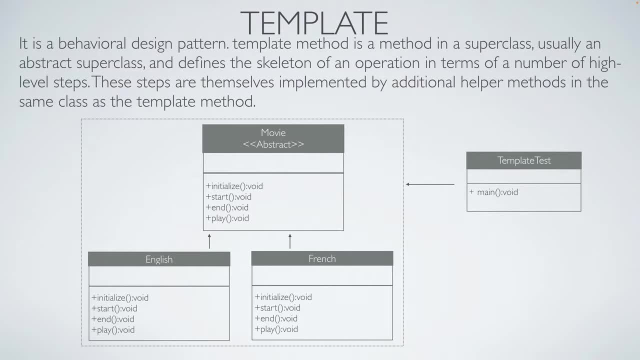 An abstract class exposes to execute its methods. Its subclasses can override the method implementation as per need, but the invocation is to be in the same way as defined by an abstract class. Let's take an example of a movie. Movie is an abstract class that has all the operations within a template method and the template method is final so that it cannot be overwritten. 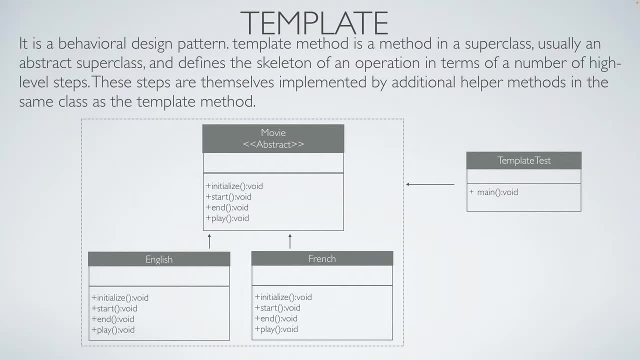 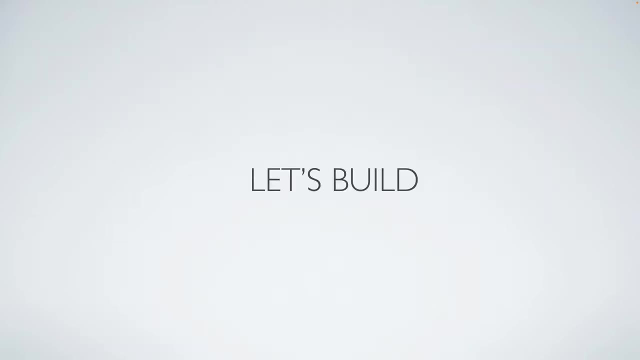 An English movie and French movie are concrete classes that extend movie and override its methods. There is template tests that will have the main method to test this feature. Let's go ahead and build this example. Let me open my Visual Studio code First. let's create a movie class. 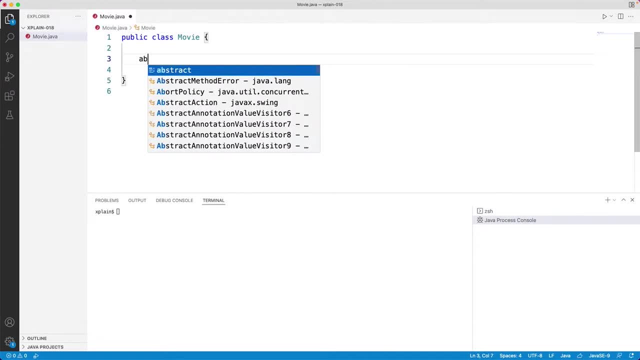 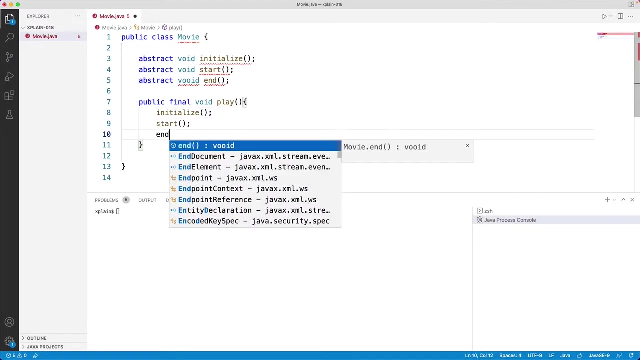 Moviejava. Within that we will have abstract void initialize method, Again abstract void start method, Abstract void end method. We will have this final method be public, Final void play. Within this we will have initialize, start and end. 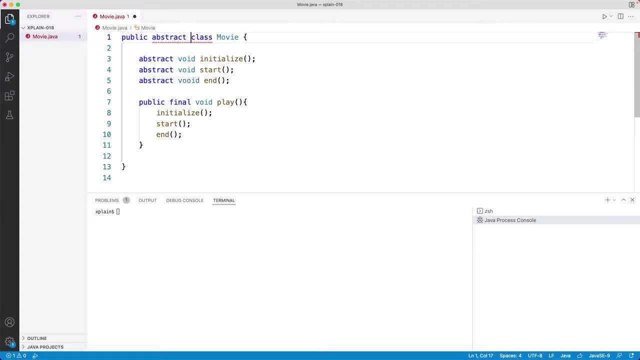 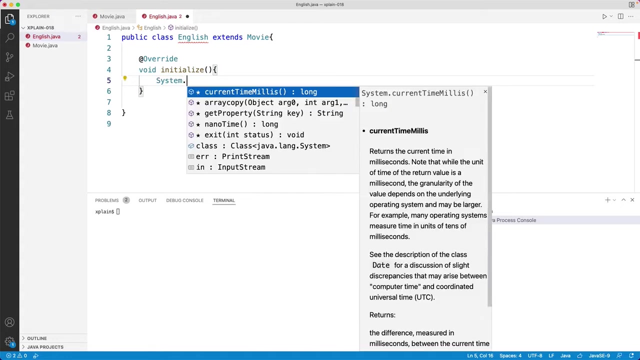 This is an abstract class. These are the methods and this is the final play method. Now let's go ahead and create an English movie. englishjava extends movie. whiteinitialize. Let's override our methods. voidinitialize Systemoutprintln. 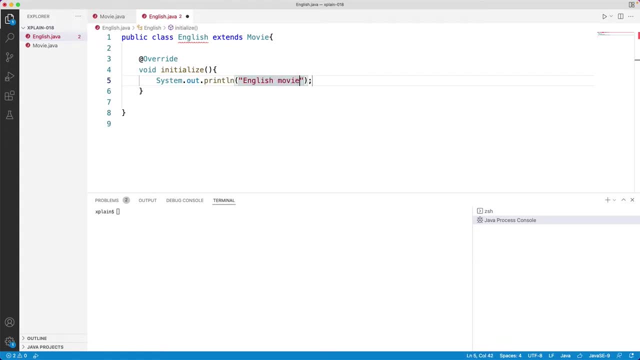 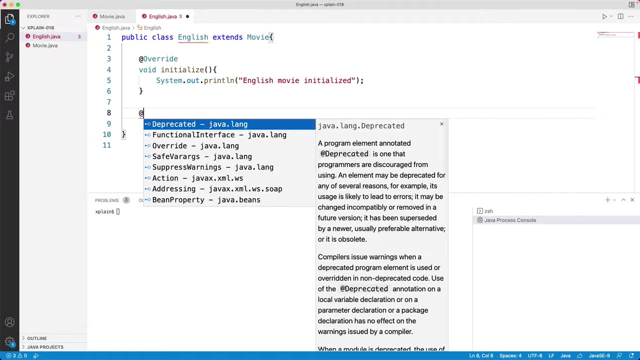 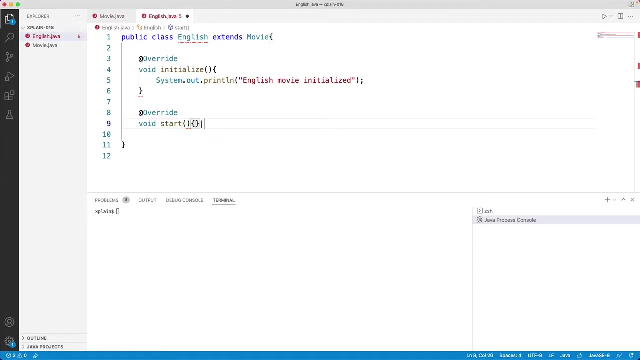 englishemovieInitialized EnglishmoveInitialize Similarly the other methods. Mathnowinitialize: override void start. systemoutprintln EnglishMovie started. and the last method: override void end and within this we will have systemoutprintln EnglishMovie ended. 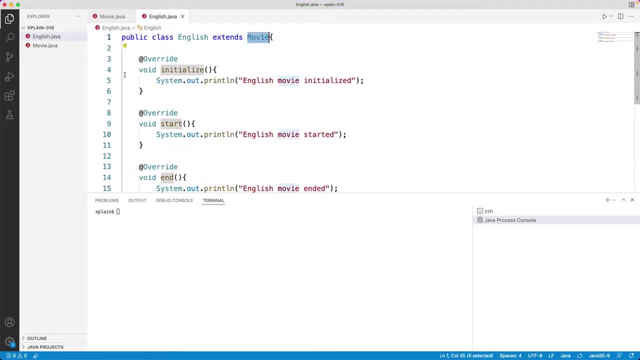 Now we have created EnglishMovie that extends movie Similar to this. let's create a FrenchMovie: Frenchjava extends movie. override void. initialize systemoutprintln FrenchMovie initialized. can override void: start. systemoutprintln FrenchMovie started. override void end. 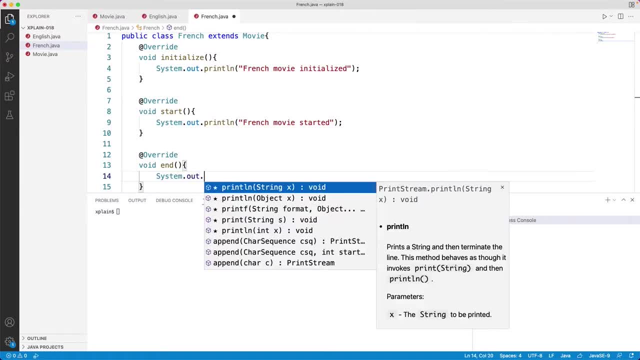 systemoutprintln FrenchMovie started and the last method, override void end and within this we will have systemoutprintln EnglishMovie started and within this we will have systemoutprintln FrenchMovie. If you see, here we have extended the movie. 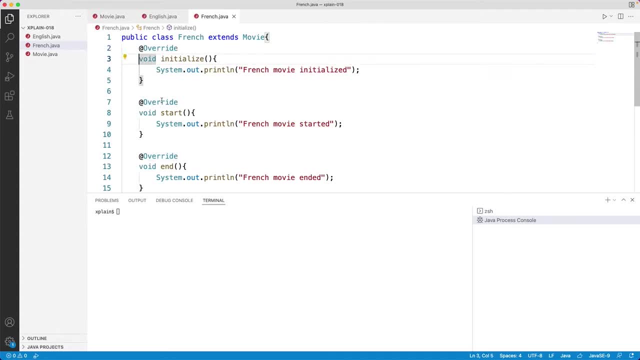 We have overridden all three methods except the play method. That is the final method. We will be using the play method to execute all these methods. Let's go ahead and create our final Preview. Preview: Preview: class template: test dot java. this will have our main method.